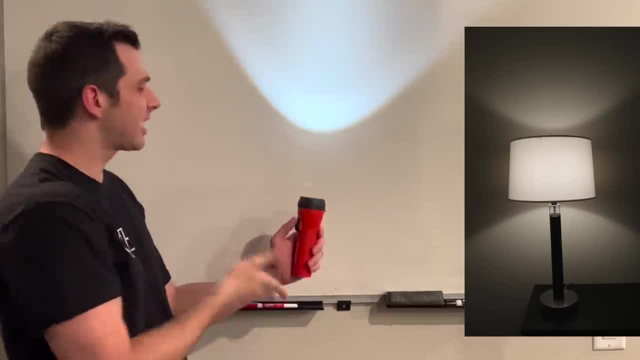 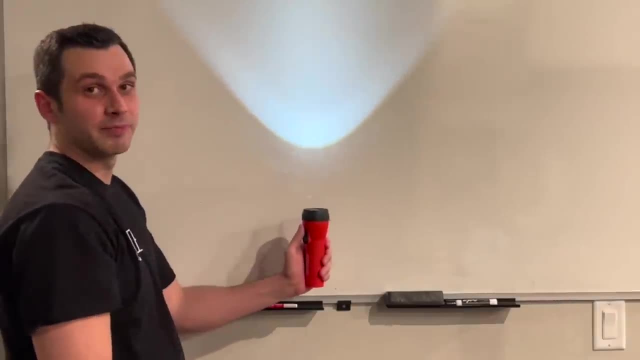 you've probably seen this a million times, because a lamp is kind of the same idea. You have a light beneath the circular hood, It's going to create a cone of light and you're going to get this shape. Now, unfortunately, I can't angle the wall. 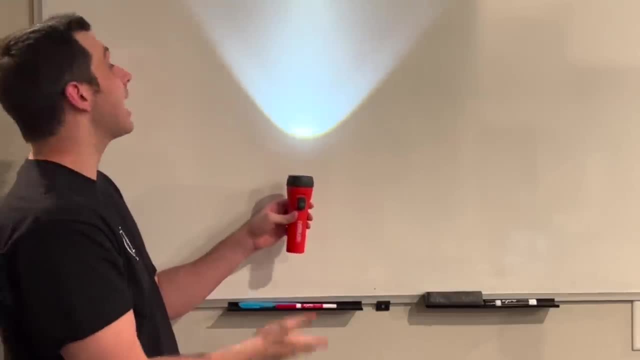 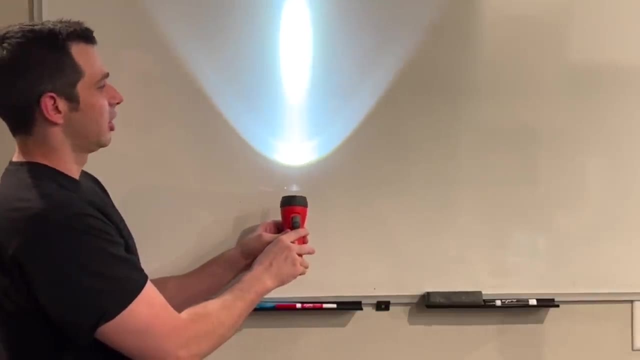 but I can angle the flashlight, The cone, So there will still be a relative angle between our plane and cone. So it's all the same thing. Now, if I angle the flashlight slightly, we're still going to have a hyperbola. 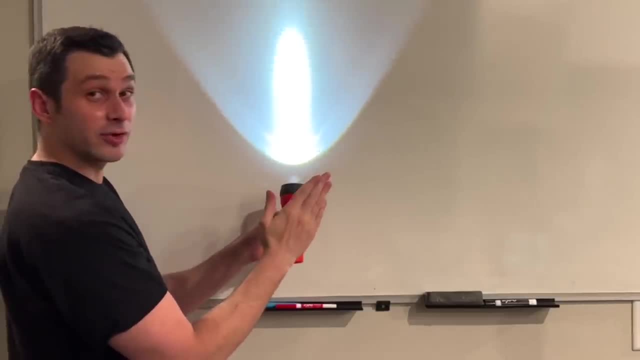 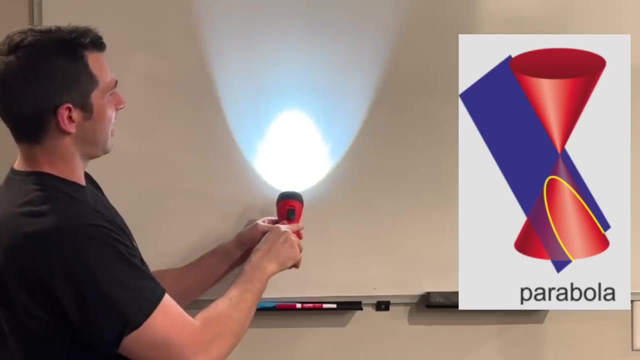 If the plane slices our cone at a slight angle from vertical, you still get a hyperbola. The parabola only comes up at one specific angle, So that's kind of hard to find, but there is one angle where you're going to get a parabola. 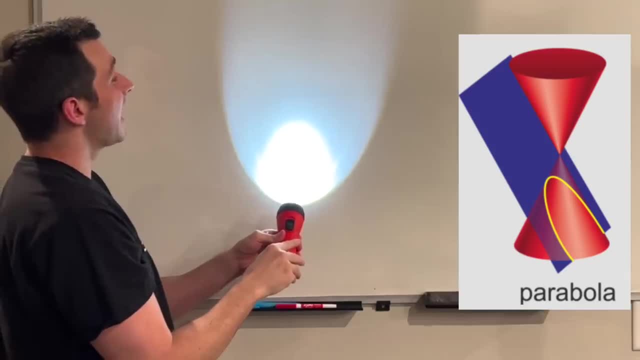 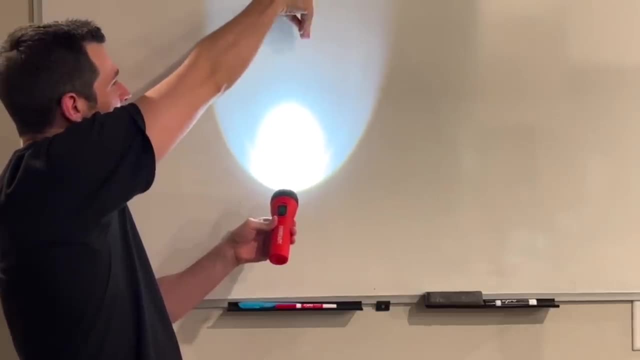 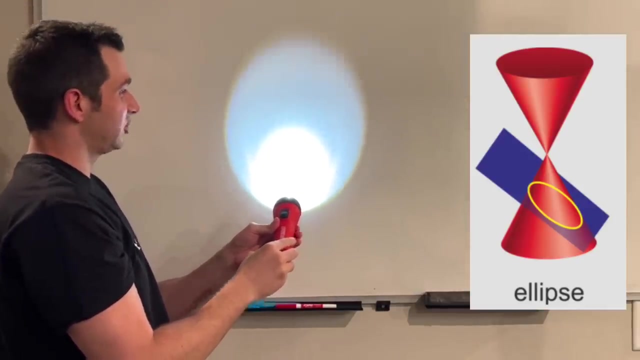 no longer the linear asymptotes. And then, if I angle it any more, what's going to happen is, essentially, the ends of the parabola are going to snap together to create an ellipse. So there we have our next conic section. And then, if I angle the flashlight straight on the whiteboard, 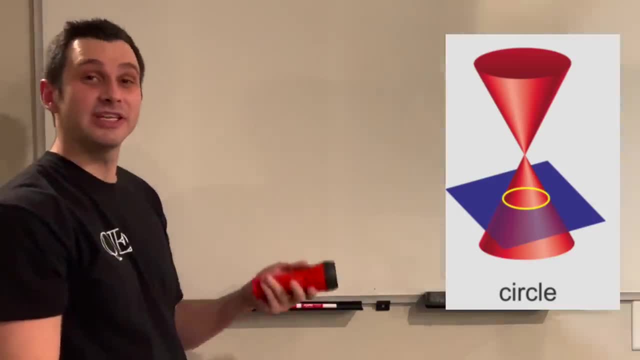 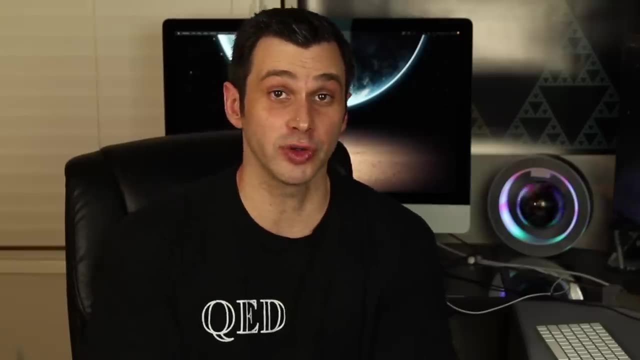 of course we get a circle. So there you go. You have seen a cone sliced by a plane before, and this was very important for what we're about to see Now. the other thing that's crucial here is we need to understand what the sun appears to do. 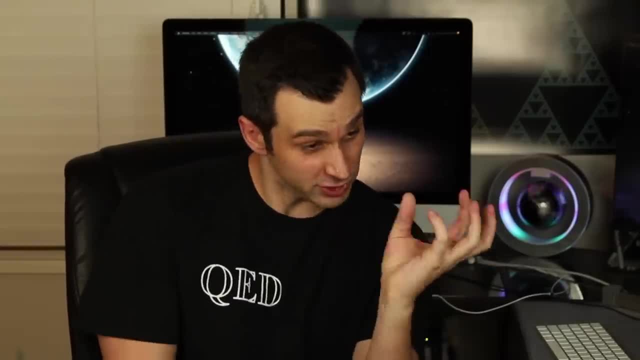 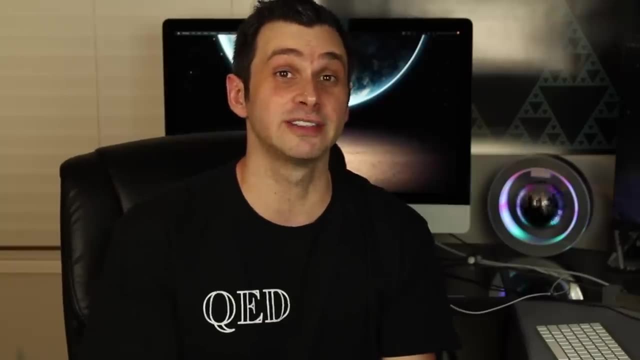 relative to us. Yes, we are spinning as we revolve around the sun, but that's not how we're going to think about this. We just need to think about what the sun's apparent path is, And that path is a circle. 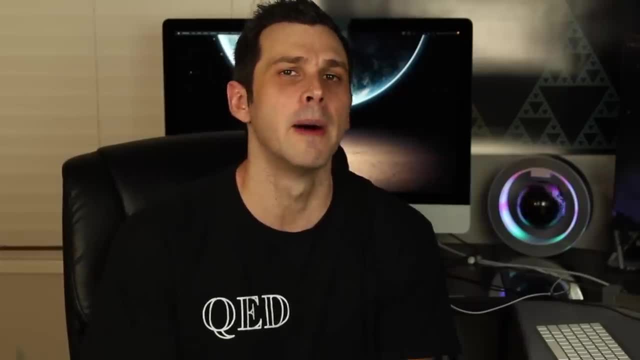 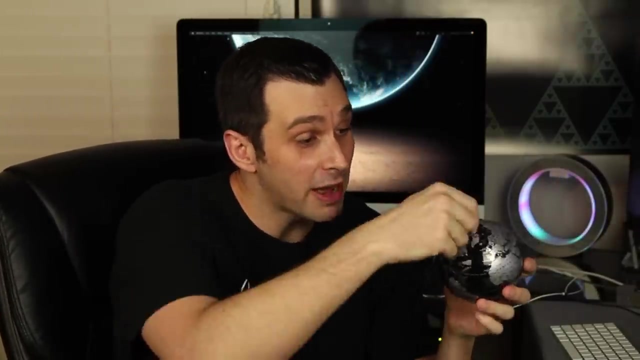 The sun appears to make circles around the Earth, But more specifically, it's appearing to make circles around the Earth's axis of rotation. Okay, so here we got the Earth chilling. Now this is the Earth of the North Pole and we're spinning about that. 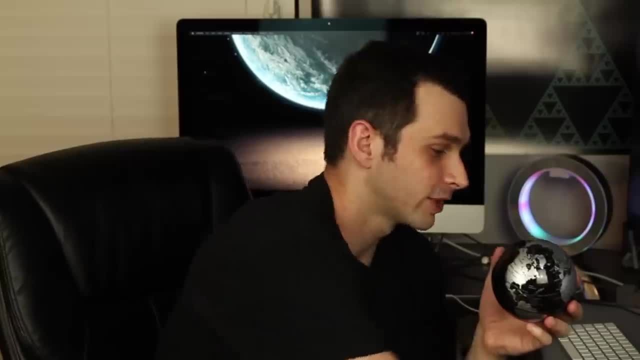 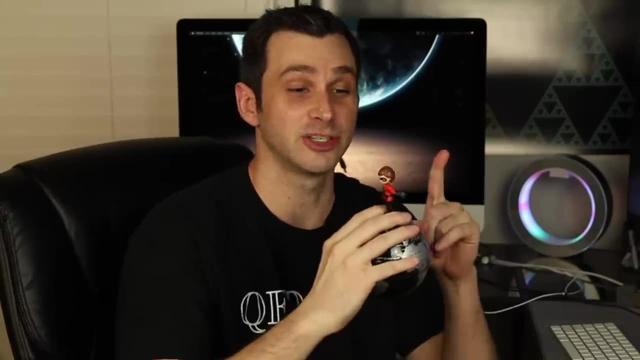 So the axis of rotation is pointing where the North Pole is pointing. If you were on the North Pole, there's you. You're on the North Pole. The axis of rotation is pointing straight up. So if you looked straight up, then the sun will appear to do circles. 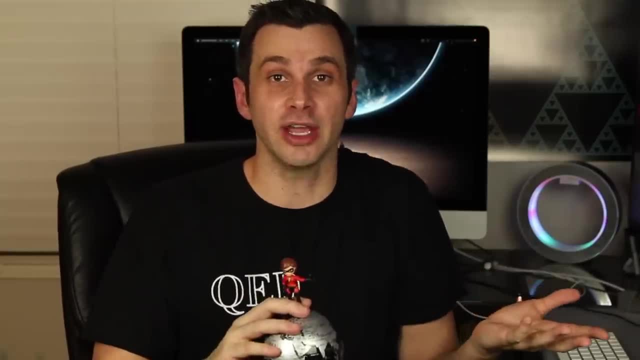 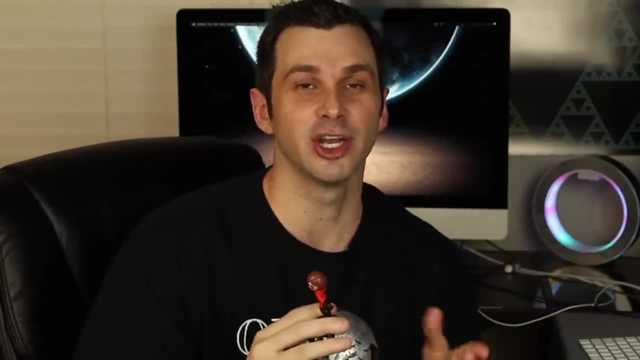 around where you're looking, that axis of rotation, That's it. If you were to lay on your back on the North Pole and just stared straight up, you would see the sun doing circles around that axis of rotation. It would never be directly above you. 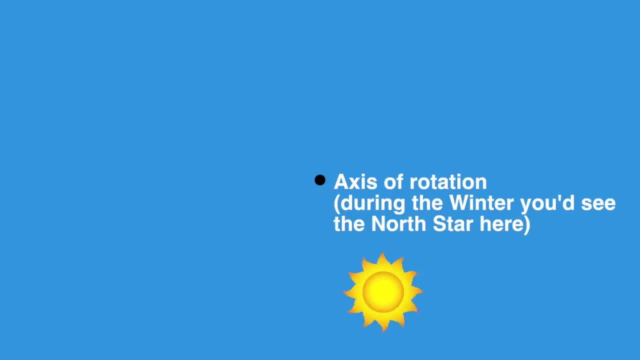 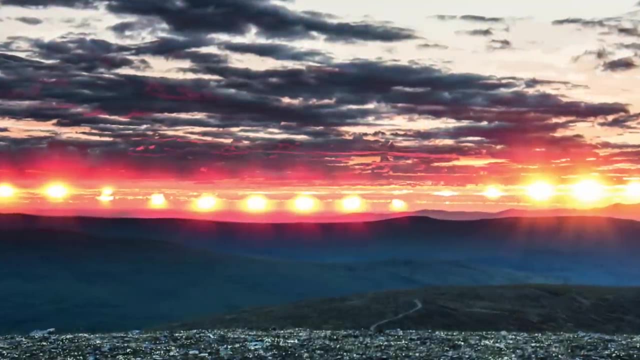 It would just be doing circles around you, assuming it was the summer. As the year went on, the circles would become wider until it went all the way around the horizon, and then it would dip below the horizon and it would be nighttime for the entire winter. 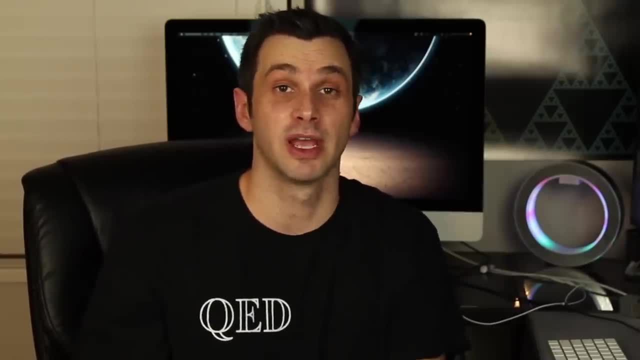 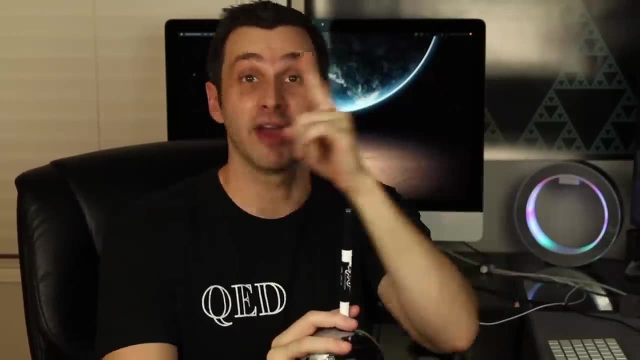 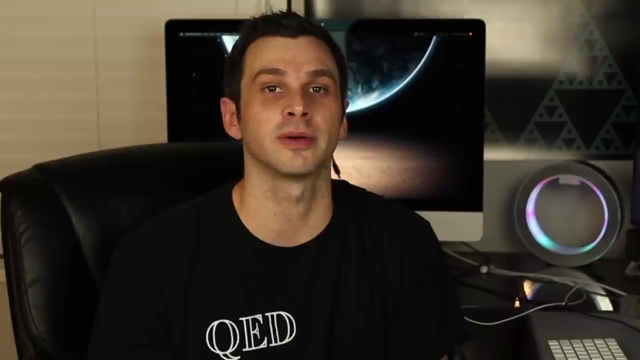 So we have one very specific answer. If you put a stick on the North Pole with the sun appearing to do horizontal circles around it, above and around it, then the tip of the shadow is going to trace out a circle on the ground. That's our first answer. 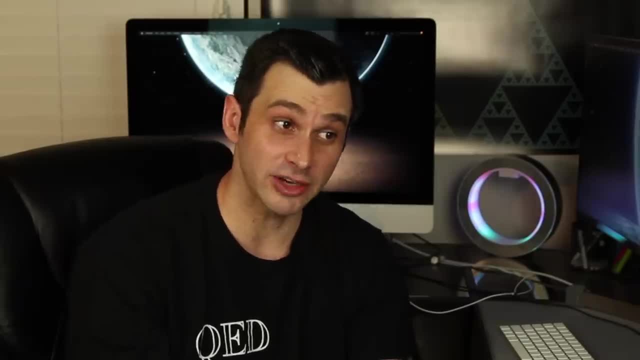 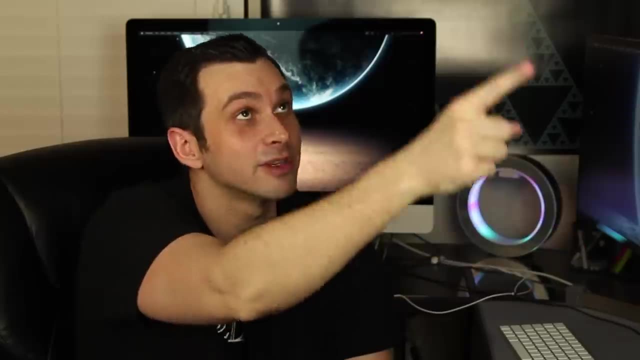 But we're not on the North Pole, So the axis of rotation is not going to be straight up. For most of us it's going to be some angle, something between straight up and the horizon, And whatever it is, the sun is still going to appear. 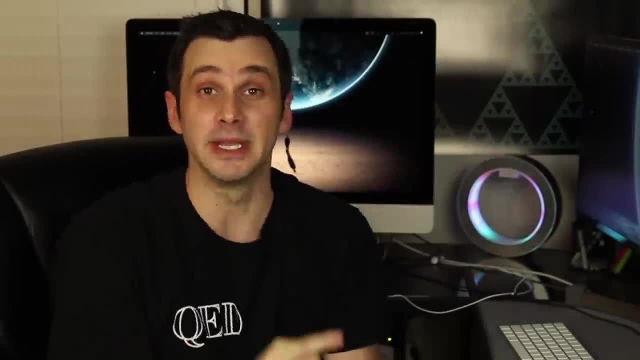 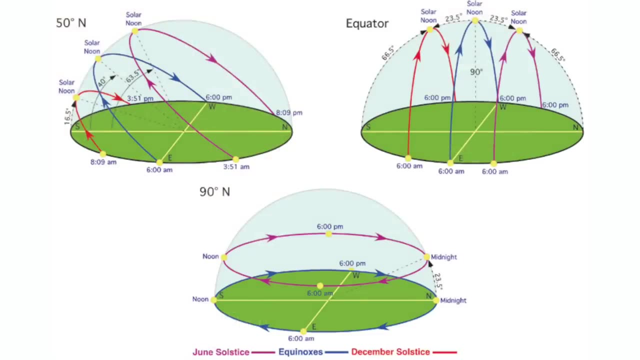 to do circles around that, But because of the angle, those circles are going to be tilted, Which you can see in this image here. Look at the top left part that says 50 degrees north latitude. This is what most of us see. 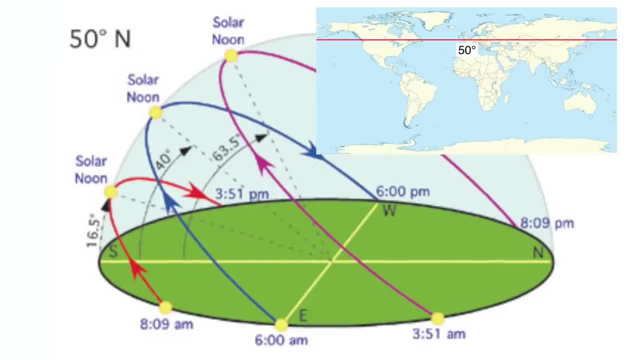 50 degrees north latitude is basically the border between Canada and the US, and it goes through a lot of Europe: France, Germany, Belgium, etc. But this is the idea for most people. The sun always appears to make pretty much perfect circles around us. 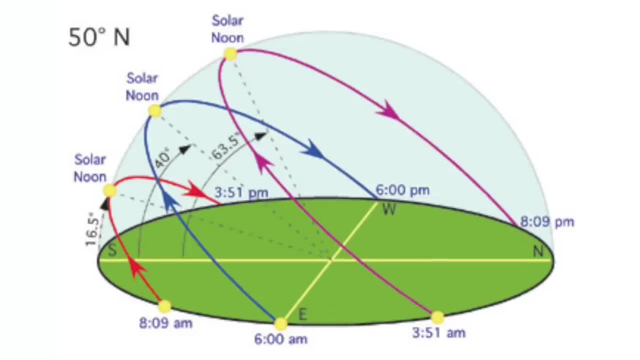 No matter where you are, But those circles are tilted for most parts of the world And different times of the year don't change the angle of the tilt for a given location on Earth, As you can see from the three different circles for the varying seasons. 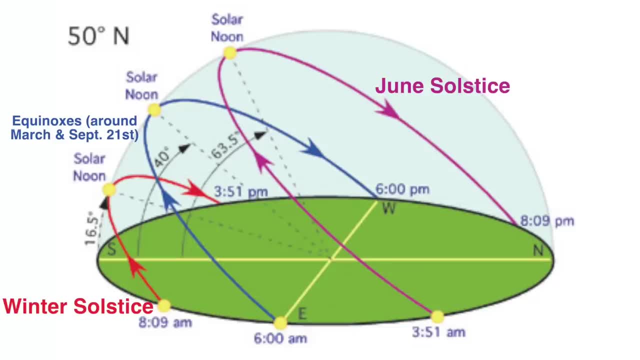 All that changes as the year goes on is the circles appear to be higher or lower in the sky. By the way, these circles are always perpendicular to the axis of rotation, So that means that axis, the North Pole, is pointing this way. 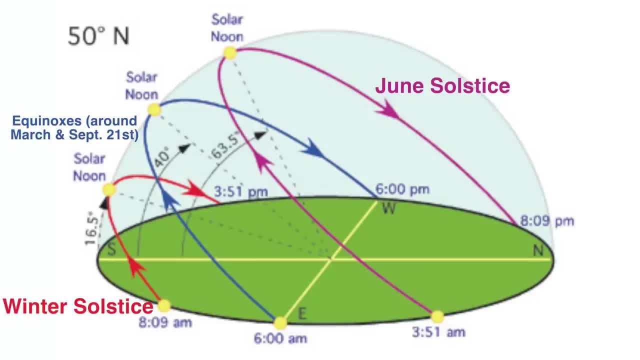 That's where you'd look to see the North Star if you lived on this latitude line. And also notice the sun only rises exactly in the east and sets exactly in the west during the equinoxes, On the bottom 90 degrees north. 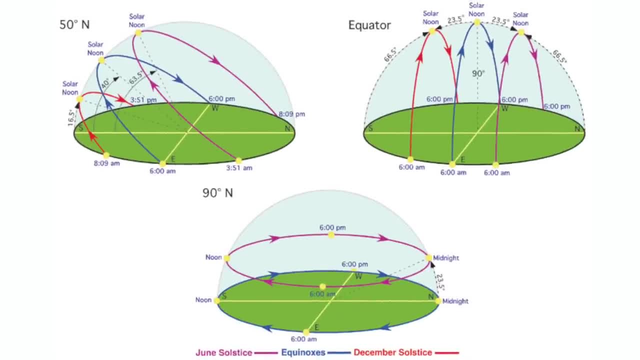 or the North Pole. we see circles that are horizontal because the axis of rotation is straight up. That's what we just saw On the equator. on the top right is where you'll find what most people probably imagine: Those actual nice arcs. 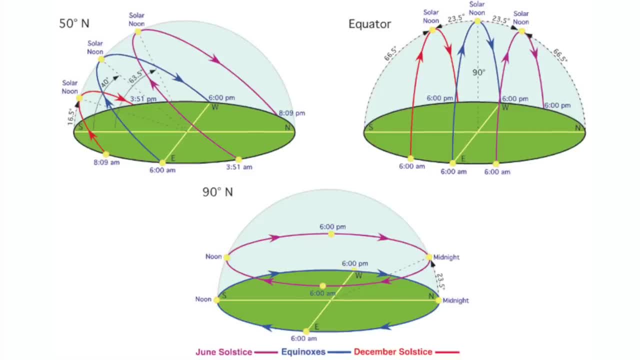 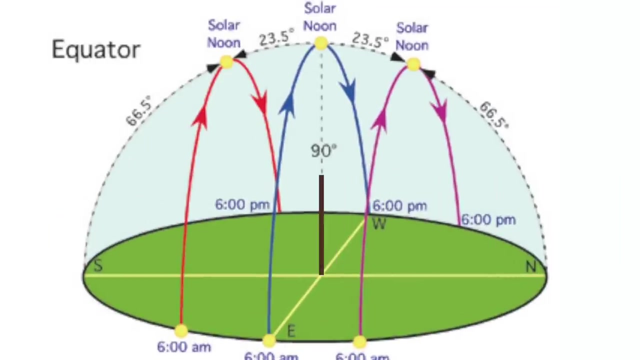 However, notice that only on the autumn and spring equinox will the sun actually be directly over your head at noon and do a perfect arc from east to west. So on those days, if you planted a stick outside on the equator, the shadow would trace out a line. 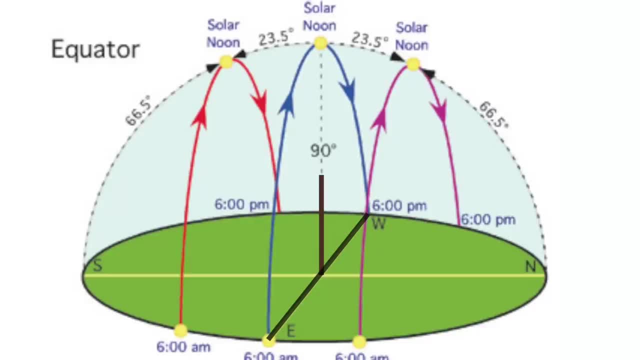 from west to east. So a line is another answer to our question, But that's only in specific cases, one being you're on the equator during an equinox, The rest of the year the sun will never be directly above your head, even at high noon. 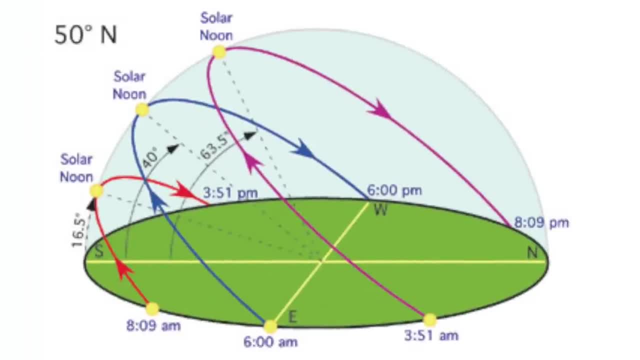 And if you live on the 50th parallel, notice that the sun is never directly above you. If you're in Seattle or Berlin and the sun is out, walk outside, point straight up and you will never be pointing directly at the sun. 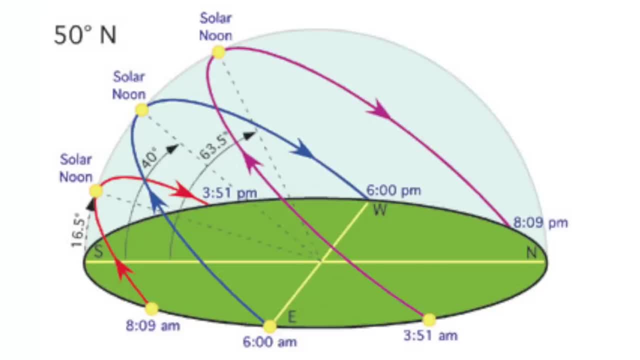 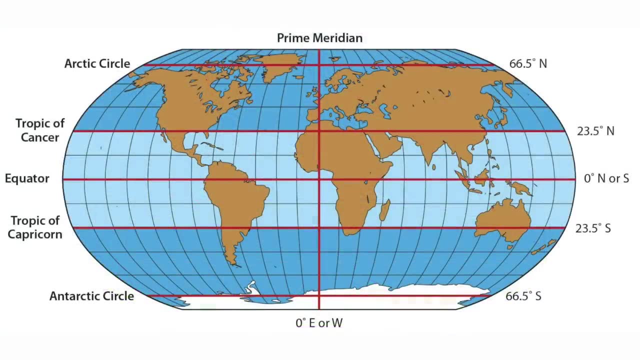 Even if it's noon on the summer solstice, You'll only ever experience the sun directly above your head if you live in this part of the world between the Tropic of Cancer and the Tropic of Capricorn. Now the vertical arcs happen on the equator. 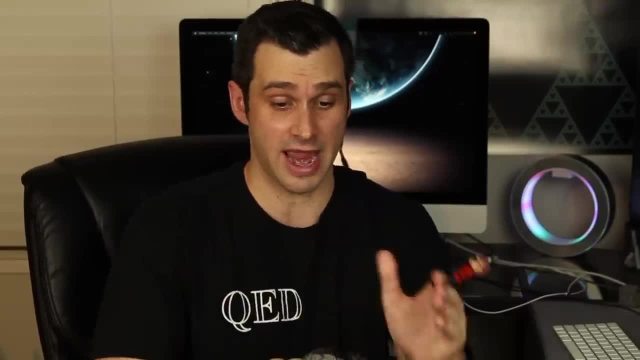 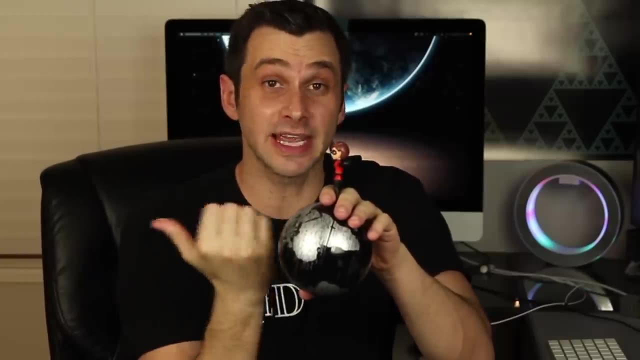 because if this is the equator right here, and that's you just hanging out looking straight forward, well, here's the North Pole facing that same direction And again, the sun always appears to do circles around that perpendicular to it. 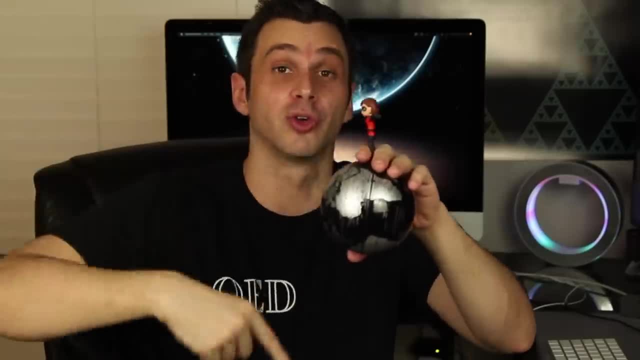 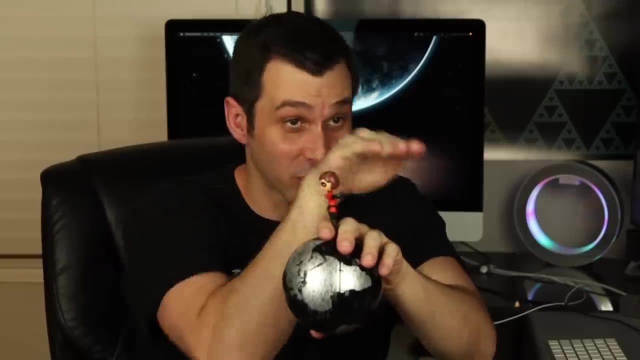 So that's why you're gonna get those nice vertical circles if you're on the equator- And it's not just the sun that does this. If you're on the equator, looking north, just at the horizon, you're looking in the direction of the axis of rotation. 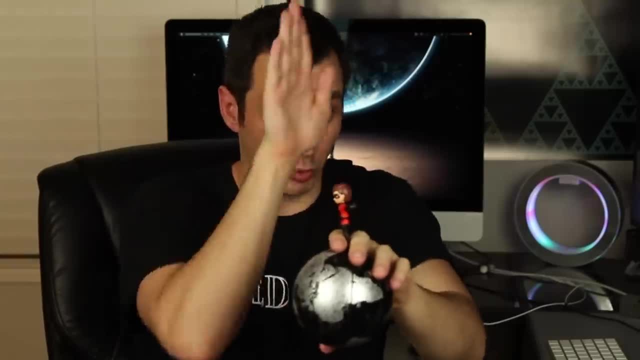 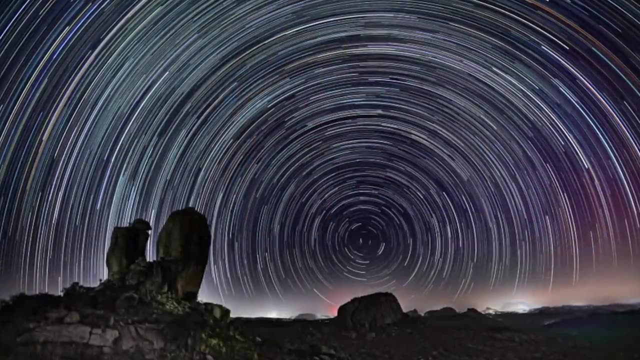 which means you're also looking at the North Star. It's gonna be right there on the horizon where the sky meets the Earth, And if you were to record the stars throughout the night, you'll find they appear to do circles around that axis of rotation. 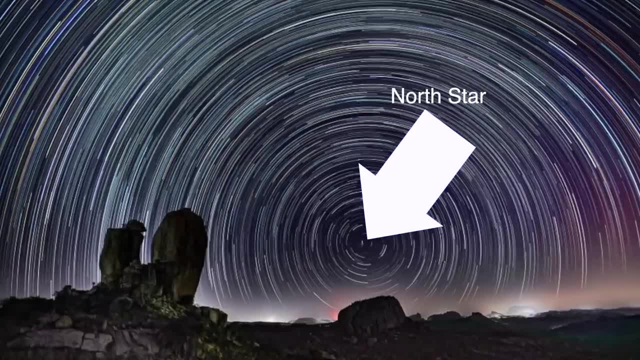 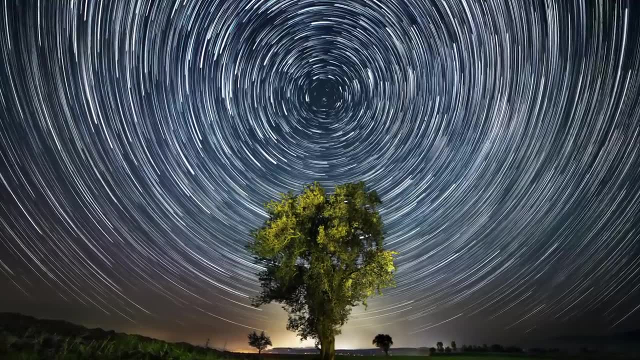 around the North Star That's on the horizon. If you're anywhere else in the world, you'll see the same thing, but that North Star will be higher up in the sky, But you'll still see those circles around it, And that's also exactly what the sun is doing. 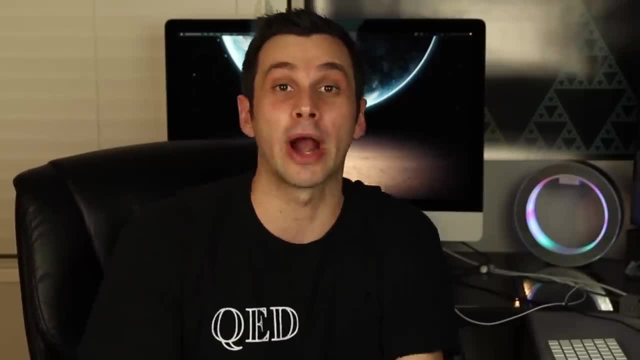 just circles around the axis of rotation or around the North Star. They're just much wider circles. And, by the way, this also all applies to the Southern Hemisphere, but you'd just be looking at the South Star. But now let's put this all together. 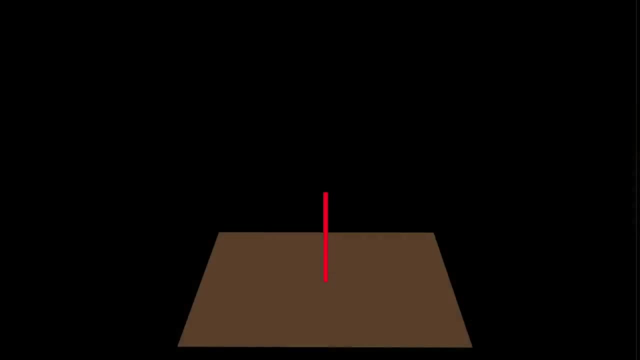 Imagine this red stick here is planted exactly on the North Pole, As we saw. that means the sun will appear to move along a circular path above it, around that axis, And to find where the tip of the shadow will be at any given point in time. 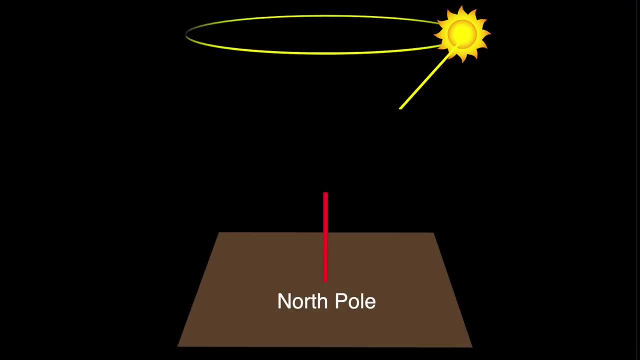 we just draw a line from the sun at that moment to the top of the stick and then follow through to the ground Wherever it hits. the ground is where the tip of the shadow will be at that time. So, as the sun does, an entire rotation. 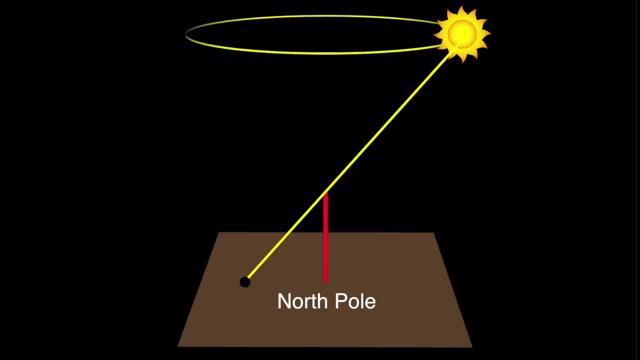 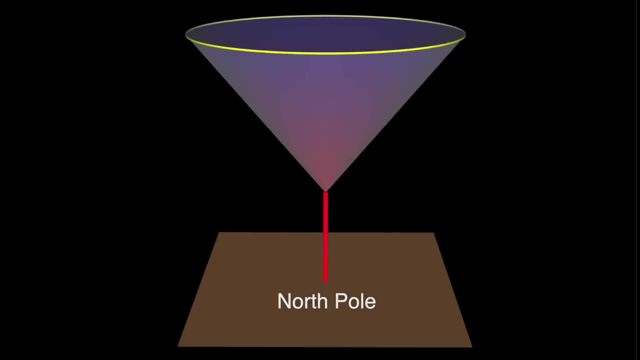 the rays traced out at each moment, from the sun to the top of the stick, will trace out- hey, look at that- a cone. And if we continue those lines through the top of the stick all the way to the ground, then we get, oh, another cone. 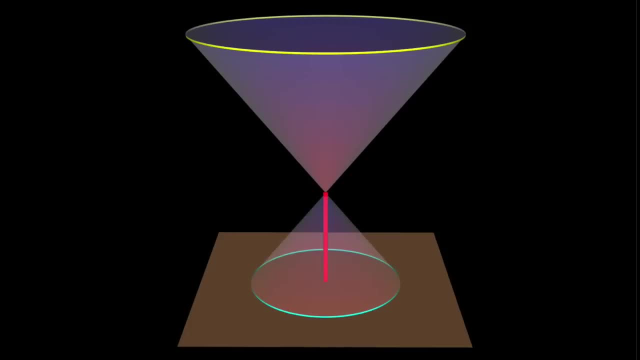 Thus the circular shadow on the ground is simply the horizontal ground intersecting a vertical cone. That's it. But typically the sun's circular path is going to appear to have some tilt to it and it will set, like we see here. 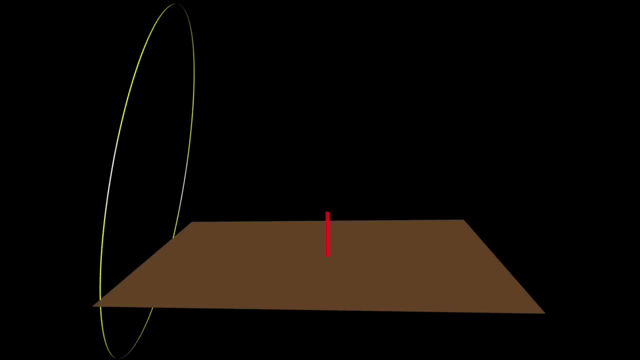 This is almost like the nice arcs at the equator, but there is some tilt. And since the sun is very far away from the earth, we can create that same cone from tracing the rays from the sun to the top of the stick for the entire circle. 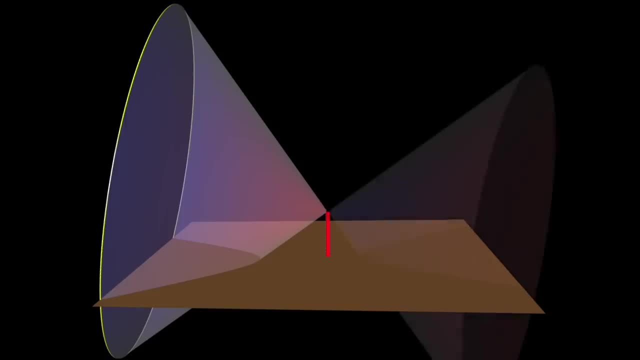 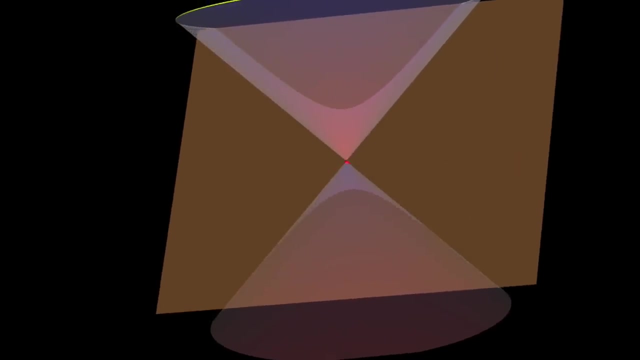 Then, following through, we find that shadow is going to be whatever shape you get, when a plane or the ground intersects a cone at a slight angle, which we know is a hyperbola, like we see here Now. it might seem weird to some of you. 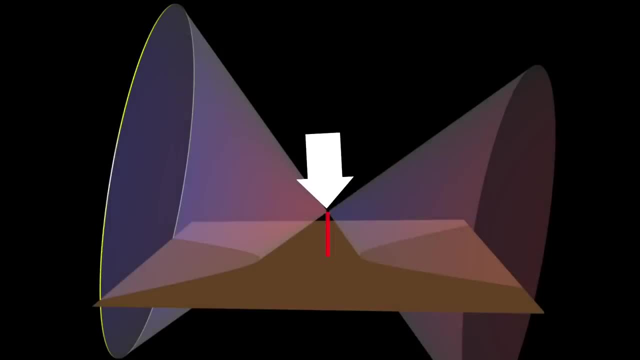 that the apex of the cone is on the tip of the stick, and you're right, It wouldn't be a perfect cone centered there, But the sun is very far away, so this still works. It is an approximation, but a pretty accurate one. 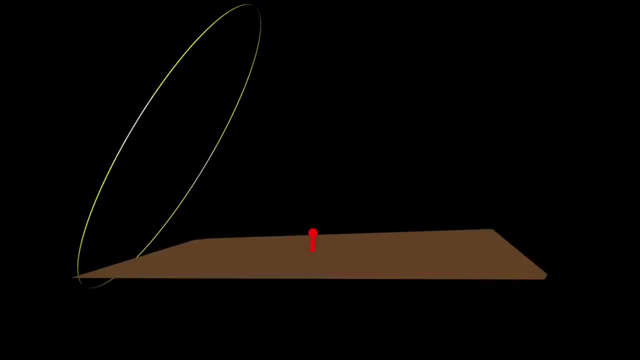 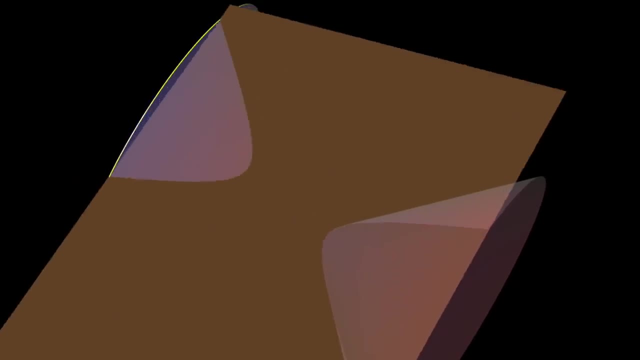 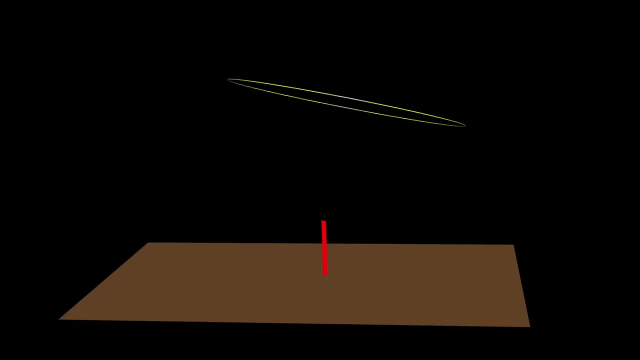 And if we're somewhere in the world with even more tilt, we need to get a hyperbola. Then we can also get an elliptical shadow. This happens when you're near one of the poles, but not on them, where the sun's apparent path is slightly tilted. 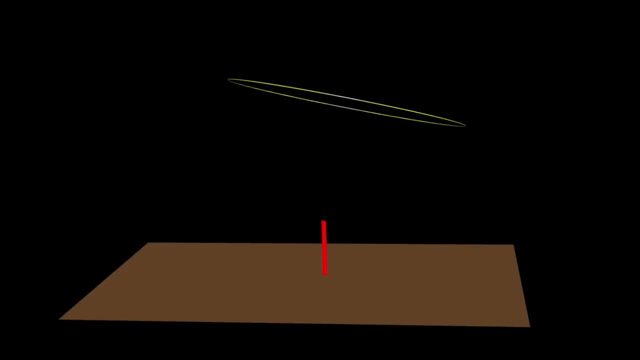 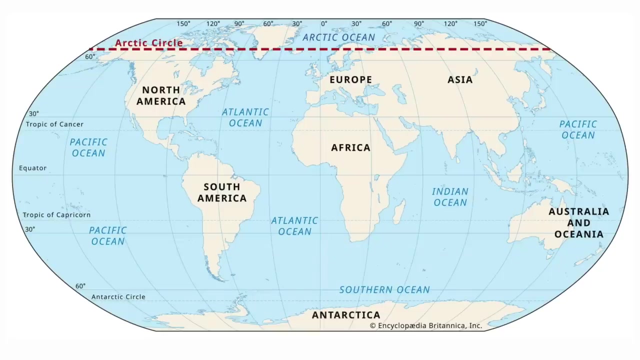 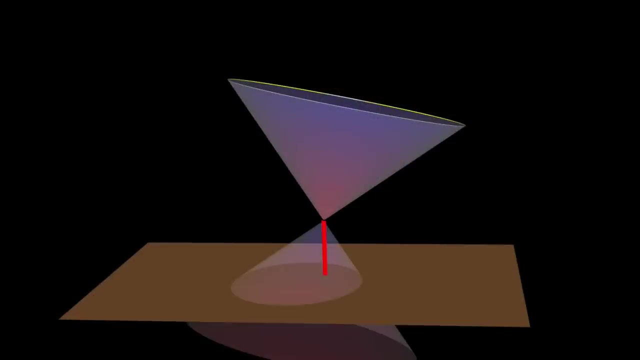 almost horizontal, but not exactly, and it doesn't set. This can only happen in the Arctic or Antarctic circles, as within those there are times of the year where the sun never sets, And during those days you will get an ellipse. 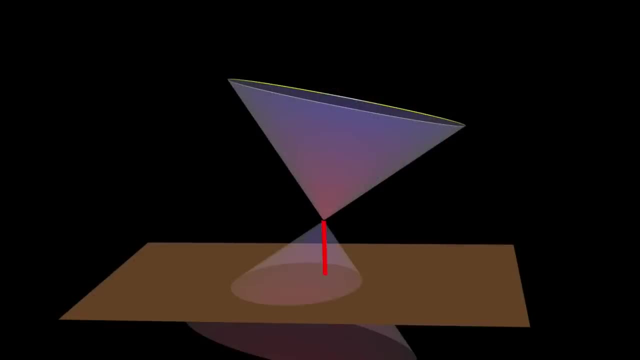 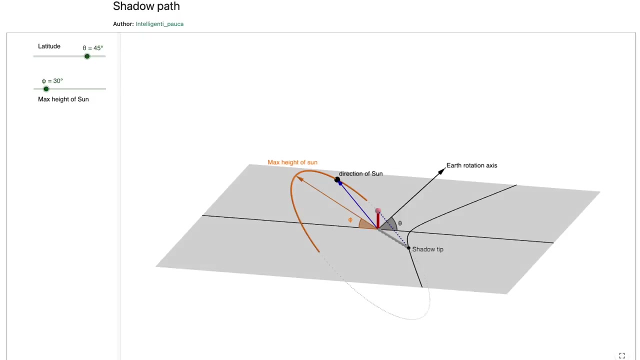 Just the ground intersecting a cone, but at a nearly horizontal angle. Someone made this nice resource here, where you can play around with different latitudes and sun locations to see how the shadow's path will change. Here's 45 degrees north latitude. 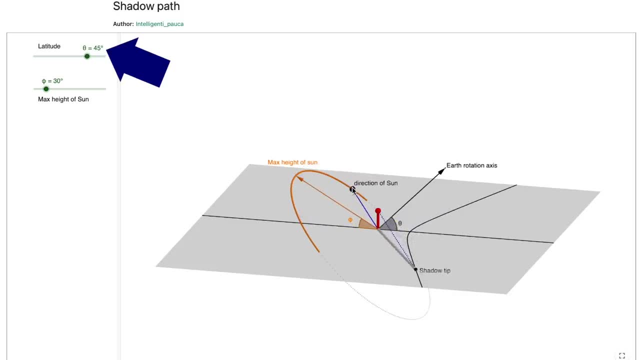 northern United States. and as the sun goes along its circular path we can see the shadow on the tip traces out a hyperbola. As the season changes, it stays a hyperbola until the equinox, when it becomes a line. 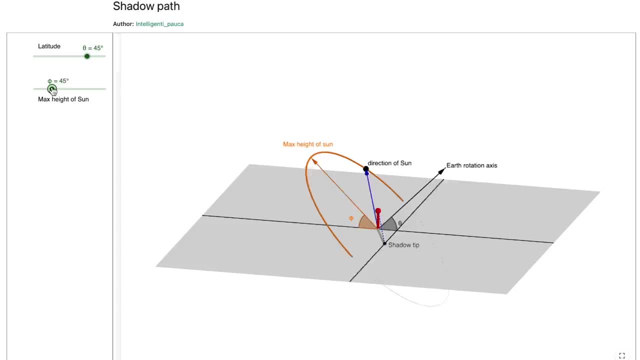 but just for that day. And then, as we move into the summer, it goes right back to being a hyperbola again, but facing the other direction. If we go to 0 degrees latitude, the equator, we again see that nice vertical arc. 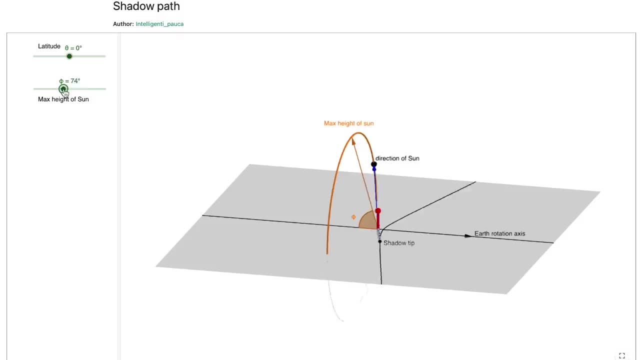 which still casts a hyperbolic shadow until again you reach the equinox and get a line. Then, after the equinox, it goes right back to a hyperbola. In fact, no matter where you are on Earth other than the poles. 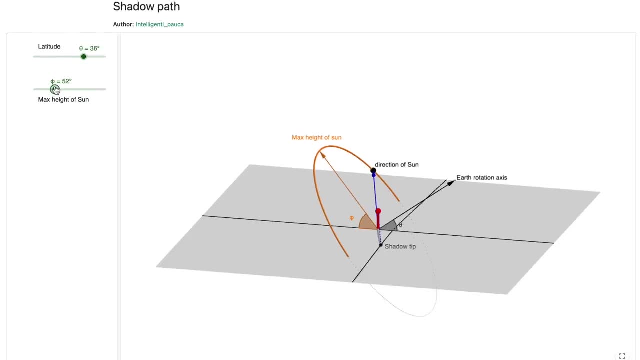 you'll find that on the autumn and spring equinox, the tip of the shadow will trace out a line from west to east. So that's the real answer in regards to the line. It will happen no matter where you are on Earth except the poles. 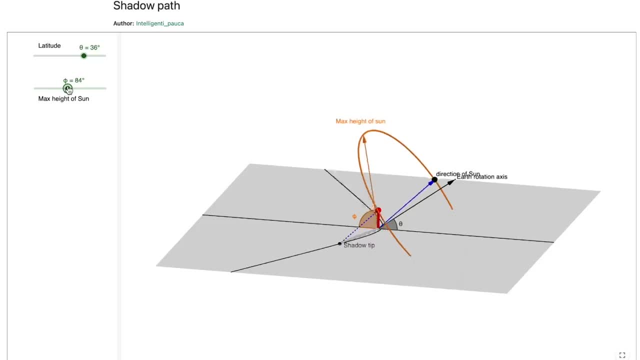 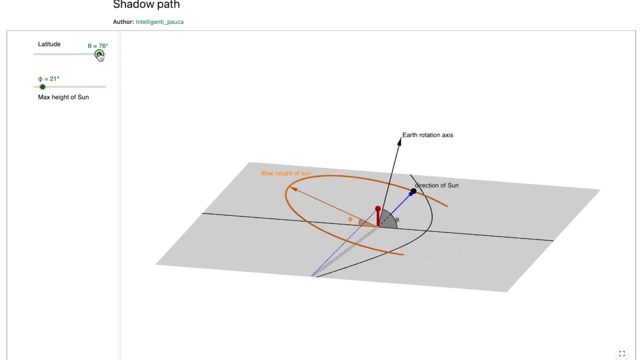 but it only happens two days a year And that's what we call a spring equinox. And the last conic section we haven't seen is a parabola, which can happen if the sun just barely sets, essentially, As in it just touches down on the horizon. 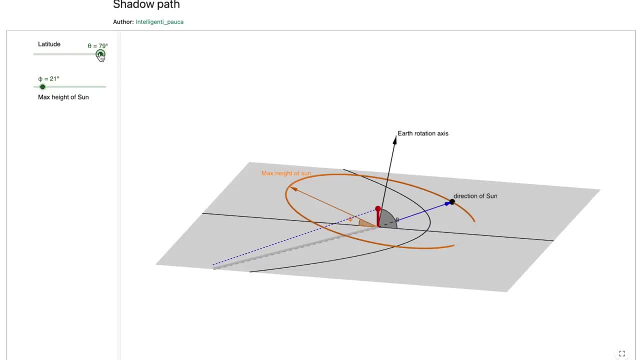 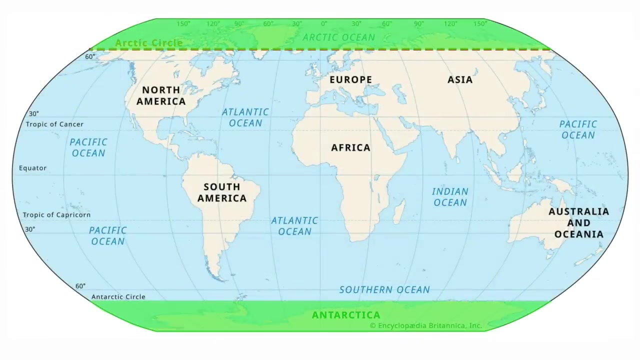 and then immediately starts to rise in the same location. That's where the shadow ends, both kind of meet at infinity before snapping to an ellipse, And this can only happen if you are in or on the arctic or antarctic circle. If you're there but not on the pole. 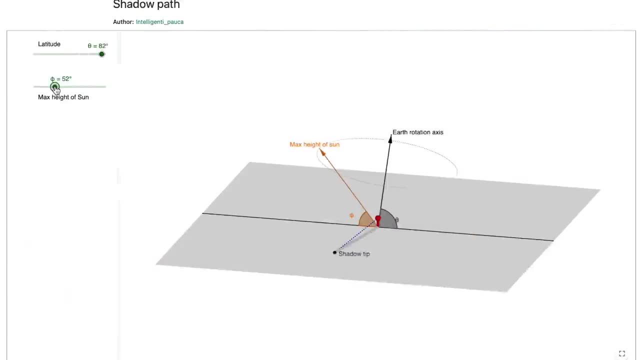 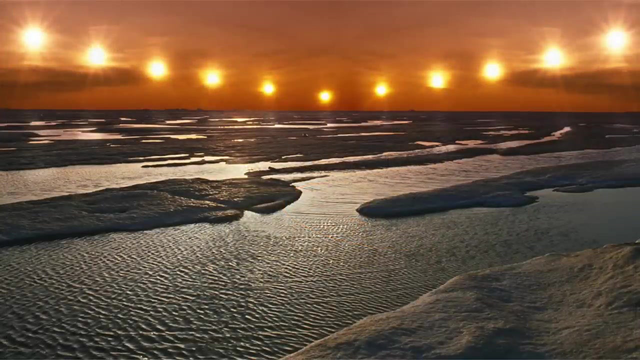 the sun will appear to have a slightly tilted circular path And as summer goes to winter, the apparent path will start to get lower and lower until one end just barely dips below the horizon, giving us that parabolic shape. Then we quickly hit the equinox. 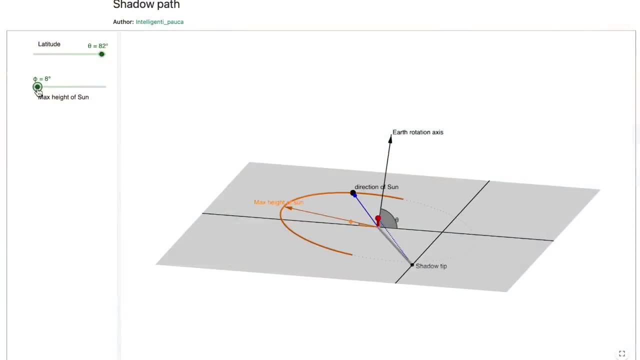 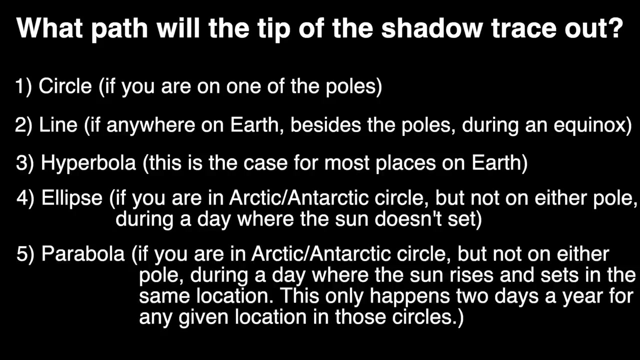 until we get that straight line shadow, and then afterwards hyperbolic, until the sun's apparent path completely dips below the horizon, leaving it dark for the winter until it comes back up. And finally, of course, the actual real world application of this. 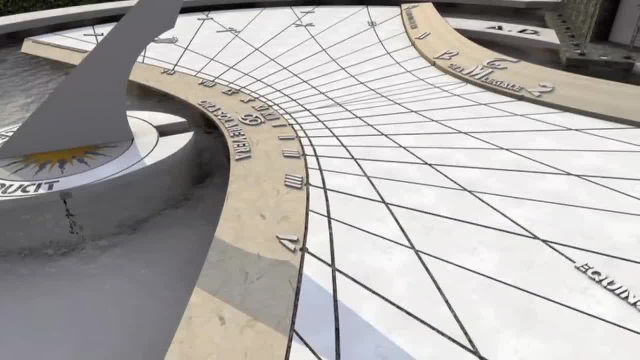 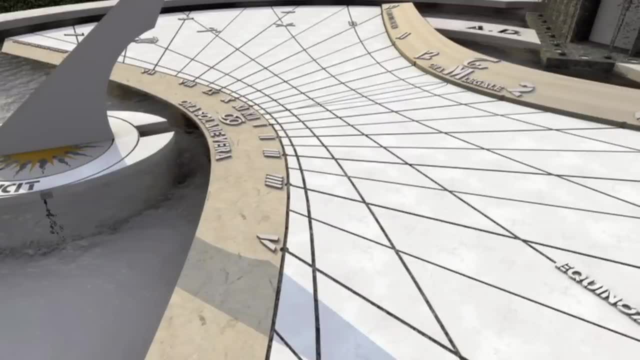 would be sundials, which do exist, based on what we've seen here, Where the path of the shadow along one of those conic sections- usually hyperbolas- tells us not only the time of day but also the day of the year. 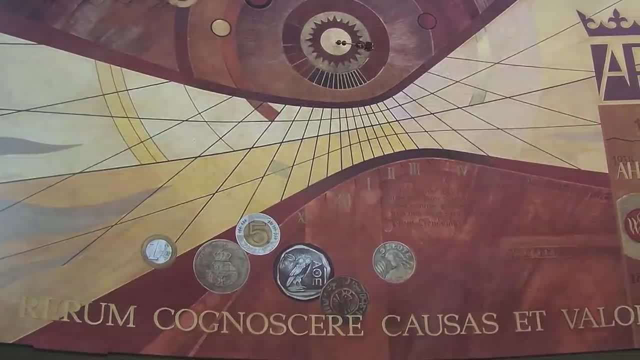 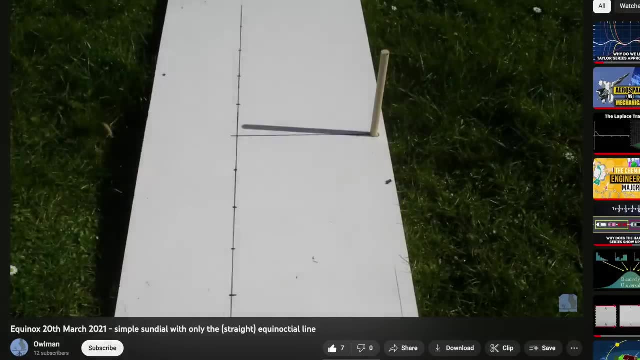 Where the more curved the hyperbola, the closer you are to the summer or winter solstice, and when you have a straight line, no matter where you are, you know it's the autumn or spring. equinox Boom sundials are cool. 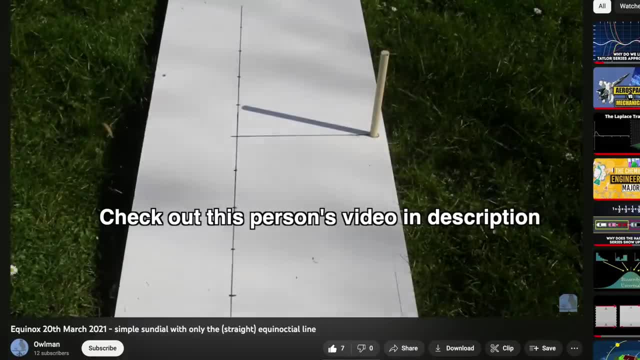 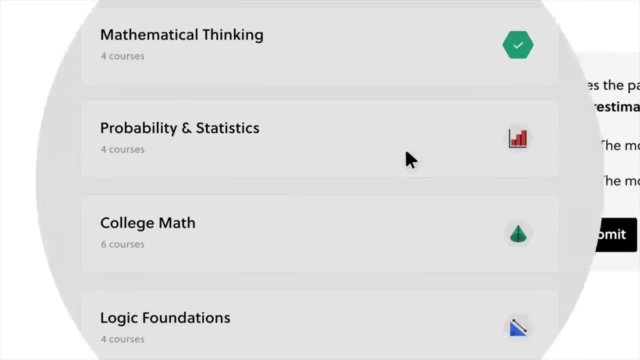 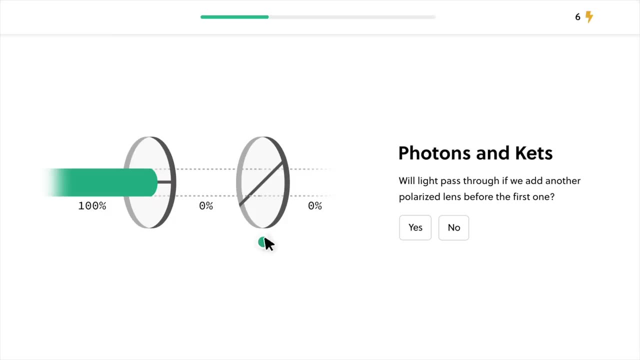 And then, before I end this video, if you enjoyed what you saw, I highly recommend checking out Brilliant, the sponsor of this video. Brilliant is an educational platform home to thousands of lessons in math engineering, with new lessons being added monthly And a big focus with Brilliant.